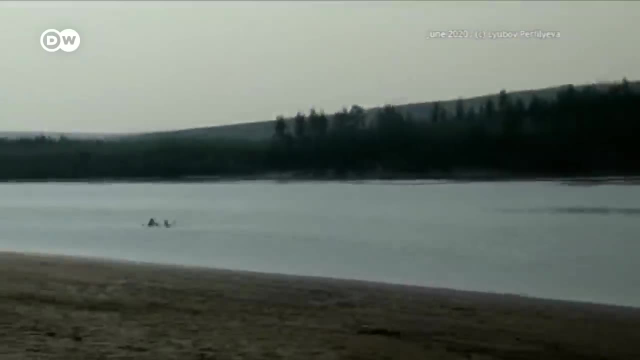 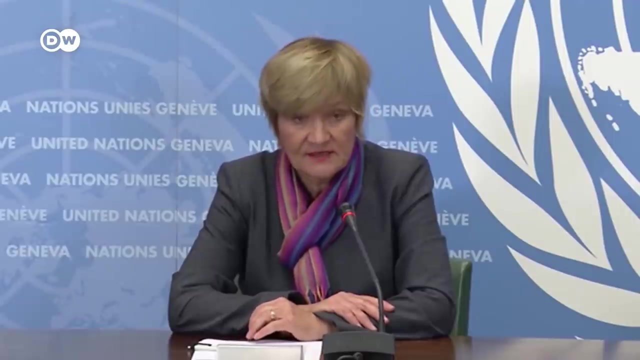 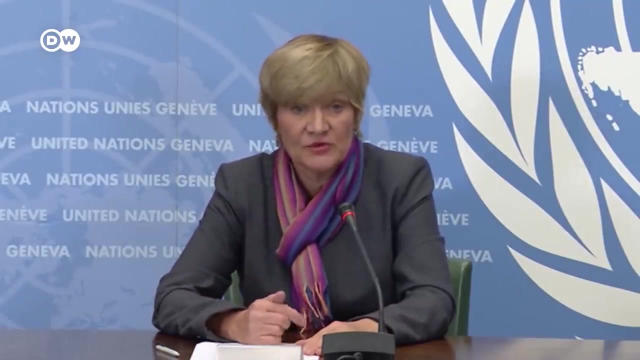 But last summer, as these images show, it set a different record: 38 degrees Celsius, The highest temperature ever measured in the Arctic. The heat that we saw in Siberia in 2020 would have been almost impossible without climate change. The Arctic, as WMO keeps saying, is one of the fastest warming parts of the world. 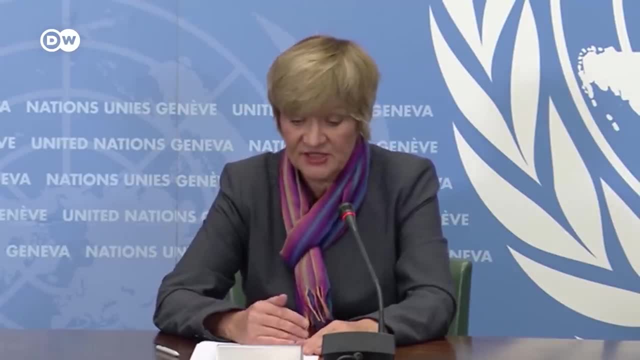 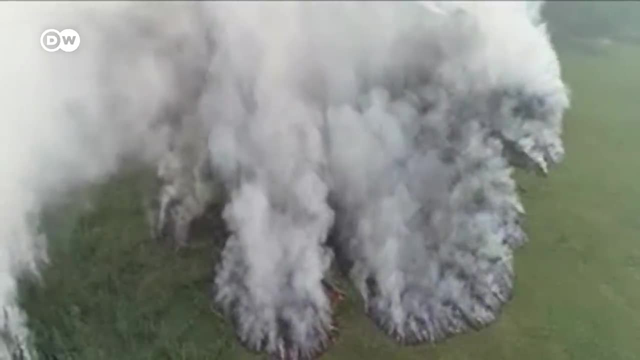 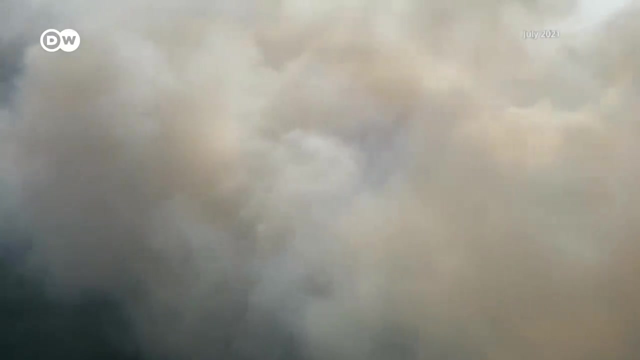 It's warming more than twice as fast as the global average, And with the heat came the drought. Even the waterlogged vastness of Siberia burned This year. according to NASA, smoke from the Siberian wildfires reached the North Pole for the first time in recorded history. 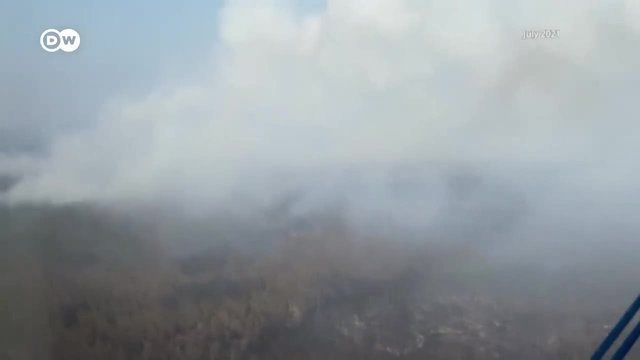 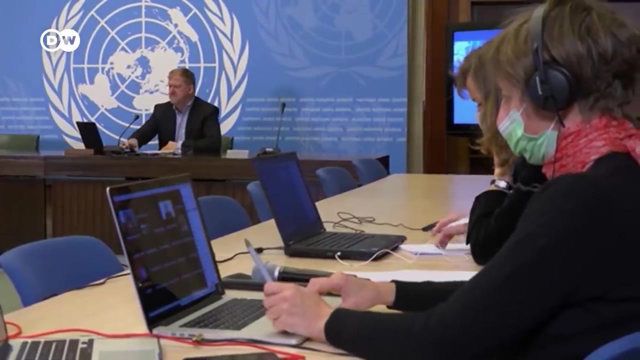 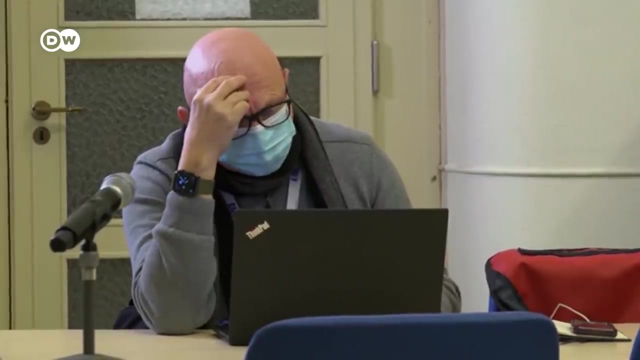 And every acre that burns releases more greenhouse gases into the atmosphere. But that wasn't the only alarming temperature record announced by the UN. This one was recorded on the other side of the globe. Last year also, there was a new temperature record in the Antarctic continent of 18.3 degrees Celsius. 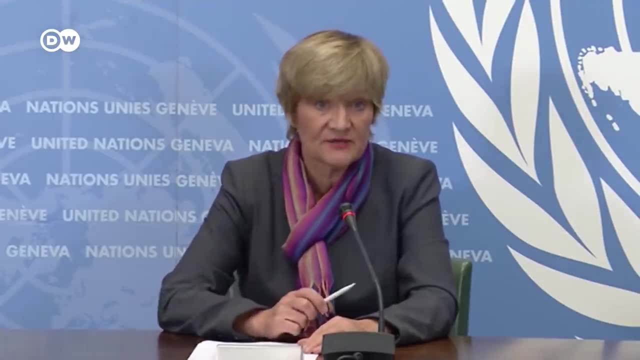 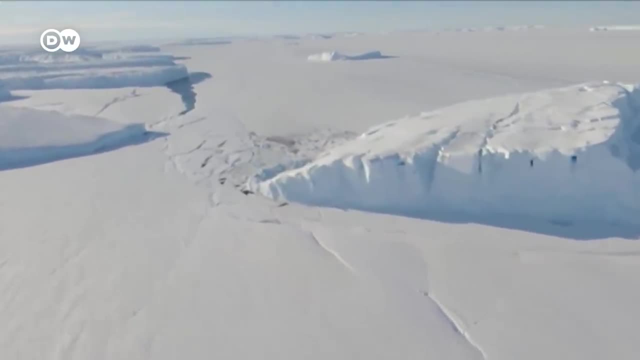 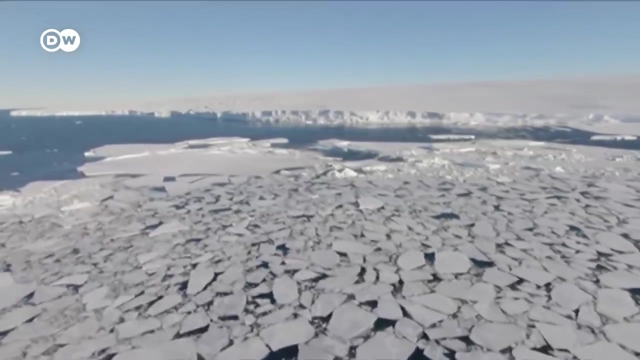 That was recorded at an Argentinian base called Esperanza. And that's not all that's happening in Antarctica. Scientists monitoring the Thwaites Glacier, which is the size of Great Britain, say it's melting so fast that it's dumping 50 billion tons of ice into the ocean each year. 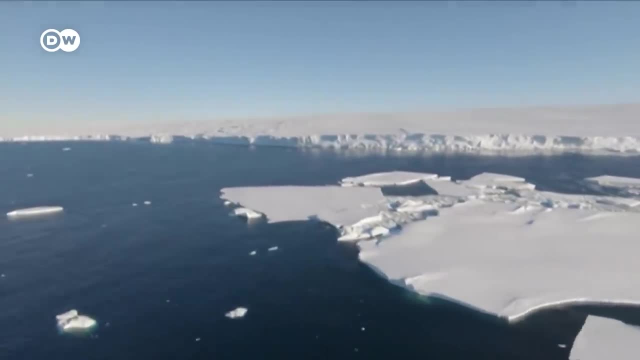 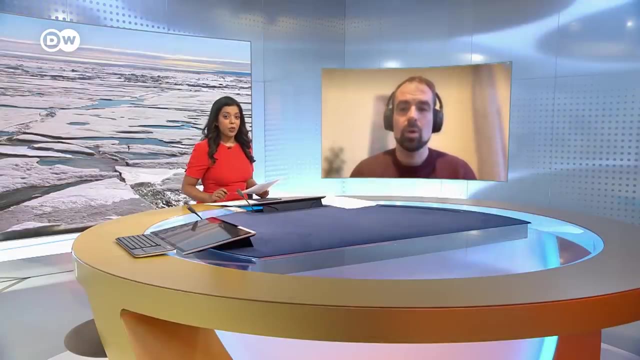 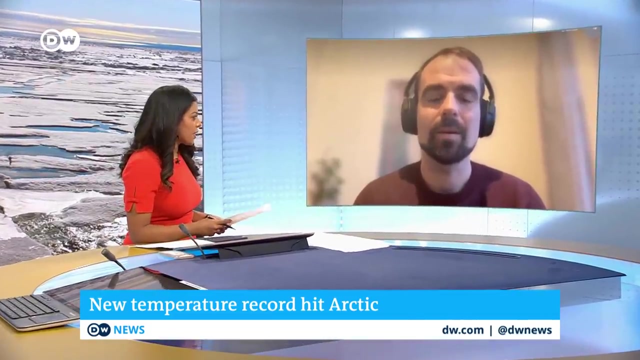 The dramatic acceleration of this melting will lead to the glacier's rapid retreat and could cause its eventual collapse. Our next guest is Carl Friedrich Schleusner. He's the head of climate science at Climate Analytics here in Berlin. Mr Schleusner, talk to us about this latest finding. 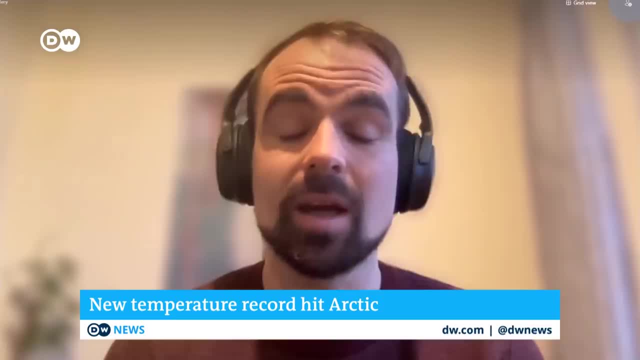 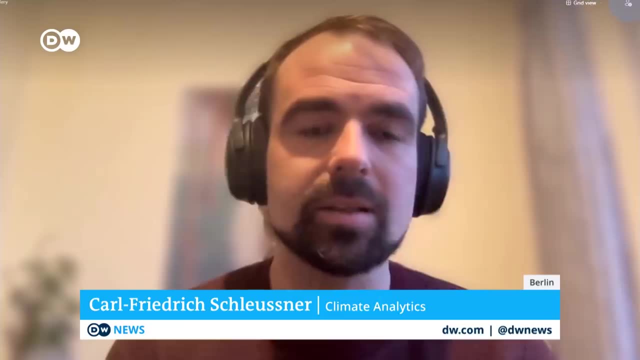 What is your biggest concern at the moment? Yeah, good morning from Berlin, And indeed it is a very concerning sign. What we're seeing there in the Western Arctic is probably the advent of something that scientists call a tipping point of the climate system. 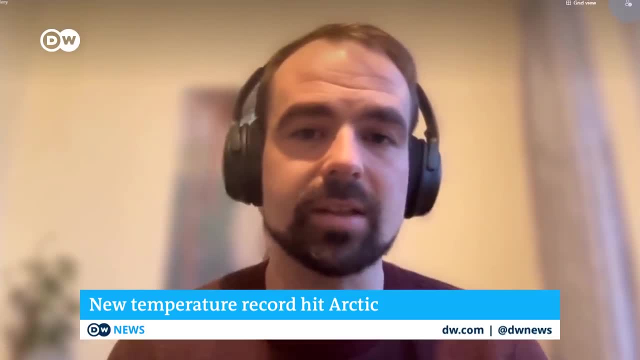 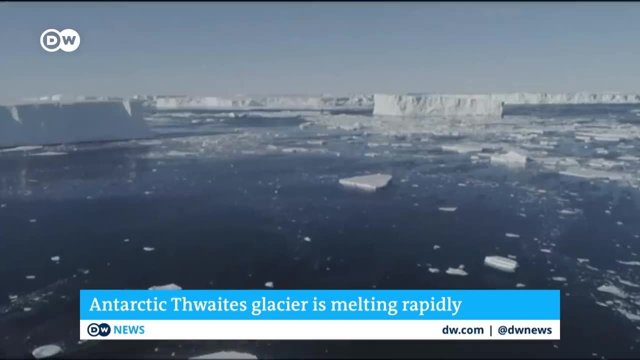 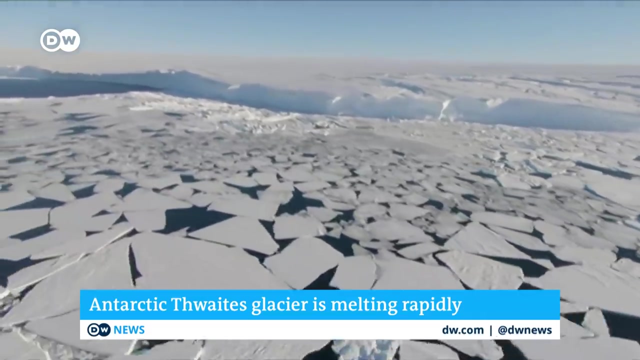 We have long been concerned about such tipping points And we know the Western Arctic ice sheet, the vast area containing ice that equates to 3.3 meters roundabout of global sea level. rise, might be destabilized if warming remains unchecked. And the gatekeeper for this tipping behavior, this irreversible retreat that would continue for centuries to millennia, is the Threats Glacier.